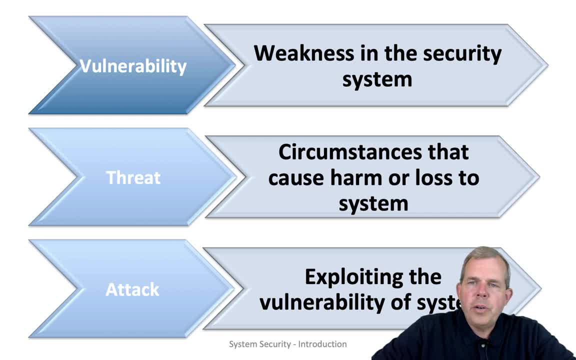 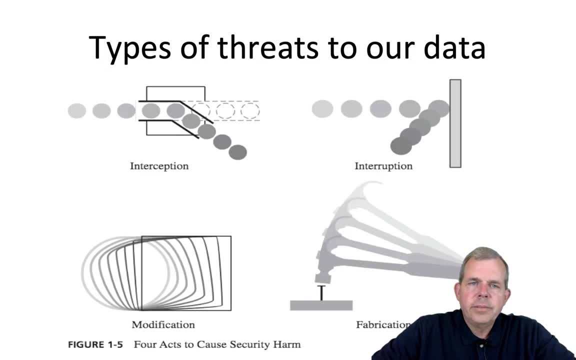 for security. I've already shown you a video on vulnerabilities in systems, and this time we're going to look at some of the things that can be threatening to your data. So really, there are just four things that were related to our threats today and, if you stick around to the end of the 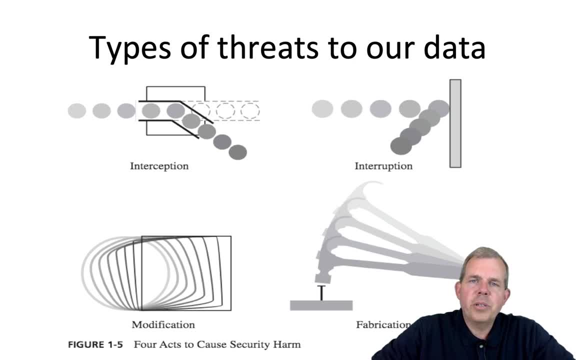 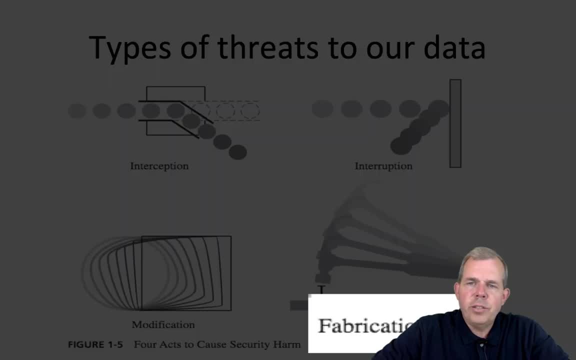 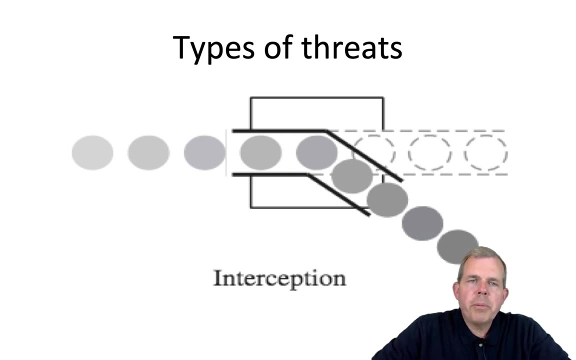 video. I'll give you a quiz and then a valuable prize if you can answer the questions correctly. So interception, Interruption, modification and fabrication are the four terms for our video. So the first type of threat we're looking at is the threat of interception. So this probably refers. 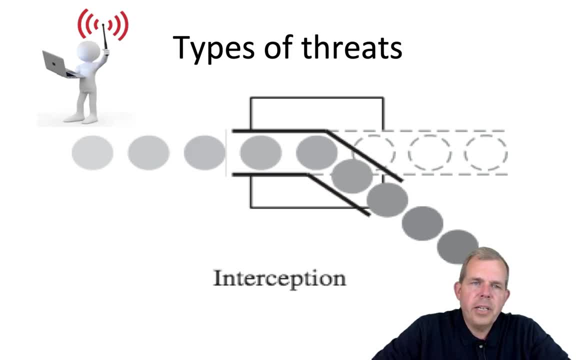 to Wi-Fi networks or anything that goes across the internet networks in general. If you were in a restaurant and you saw this on your phone that says: choose a network. it is a free Wi-Fi connect. Why not? What could go wrong? 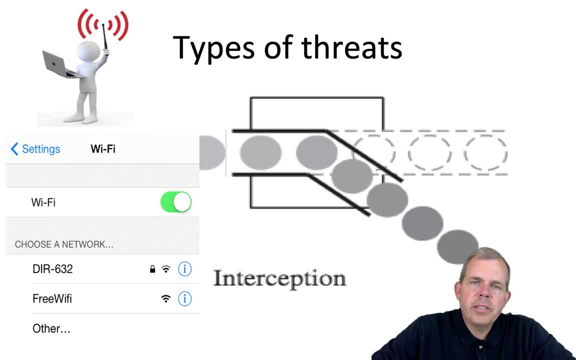 Well, what could go wrong is that somebody could set up a Wi-Fi access point that serves you the pages you look for, but also looks at all of the data that passes through Your login name, your password, credentials for things, what you're. 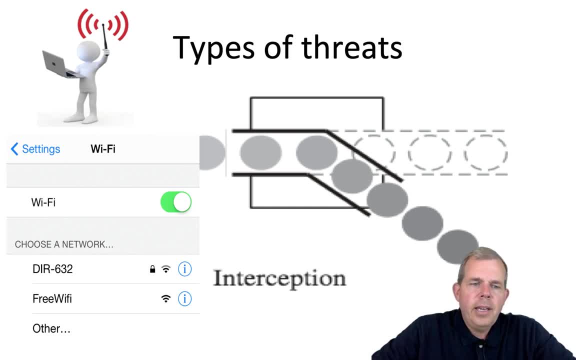 buying, what connections you're making to which websites, and you would never know it, because it just passes through the system and onto the internet. That's called a man-in-the-middle attack and it's one of the easiest ways for people to steal data. 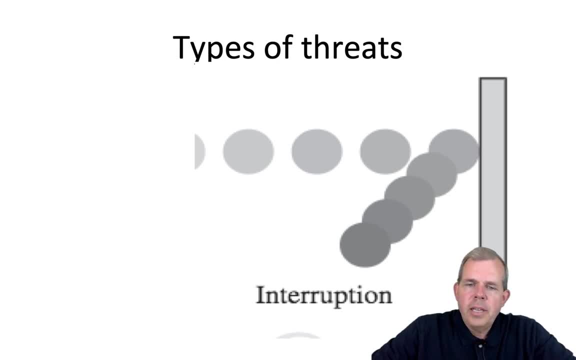 Another type of attack could be what we would say is an interruption attack, And so this brings a system down. If you were to look at a website one day that says the system is unavailable, or something similar, it could be that they're under attack. This attack is usually called a denial of 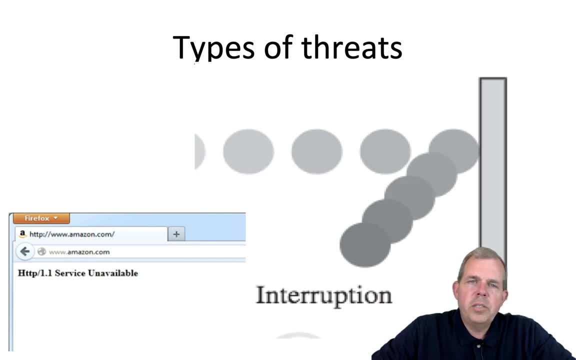 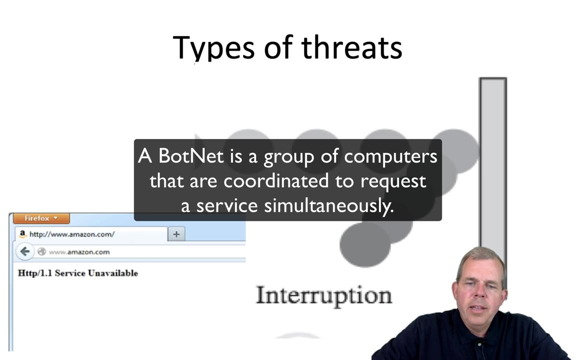 service attack or a DOS. It really doesn't steal any data, but it can damage a business by making its services unavailable. What this is usually accomplished is by maybe thousands or even millions of computers that simply overwhelm the ability of a computer response, And so a denial of service is an 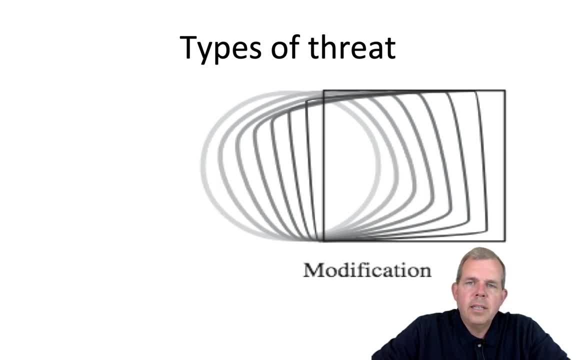 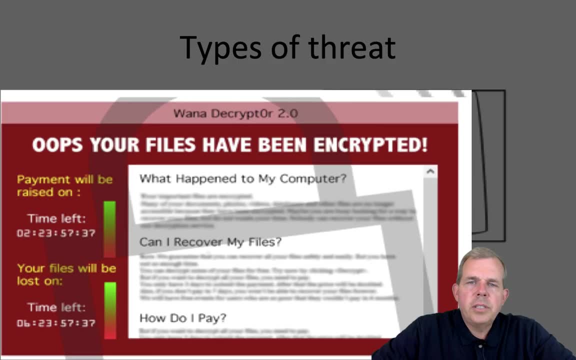 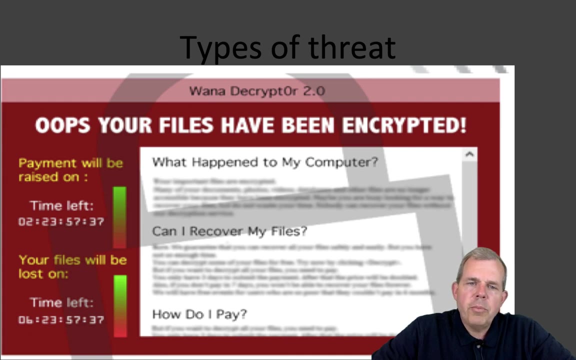 effective threat that's very difficult to defend against. A modification threat would be the next category. So you may have heard a few years ago of a system called the WannaCry virus. WannaCry was like a Trojan horse program. It slipped into your computer. It looked good, but it would quickly encrypt the entire contents of your 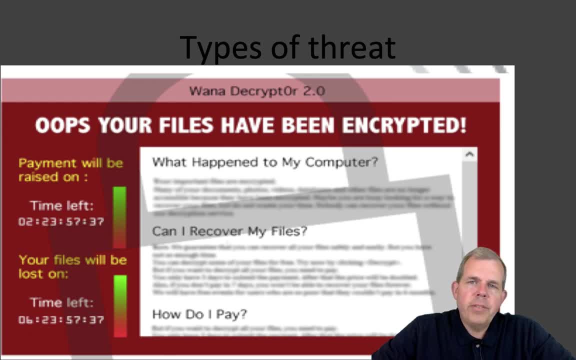 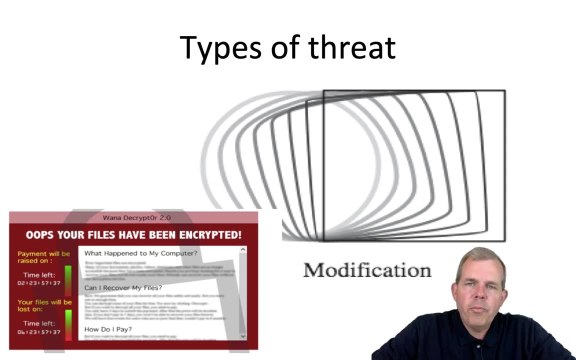 hard drive, And so an encrypted hard drive is unreadable. Your data was essentially lost. It was held hostage And you would pay some money in Bitcoin, and if you didn't pay, the program would simply erase your hard drive, As I recall. 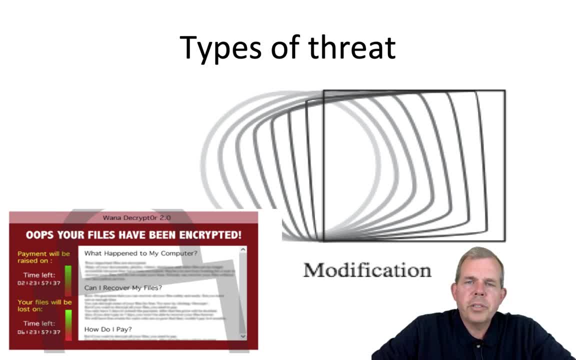 it seemed like hospitals in the United Kingdom were especially threatened or attacked by this system. So many people had to pay out money to the hackers and I don't believe anyone's ever been caught or charged or even convicted of the WannaCry attack. Millions of computers, apparently, are still. 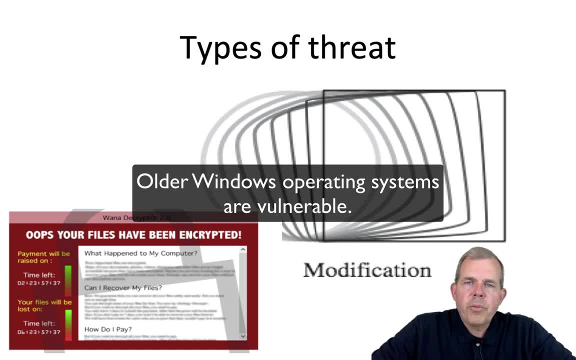 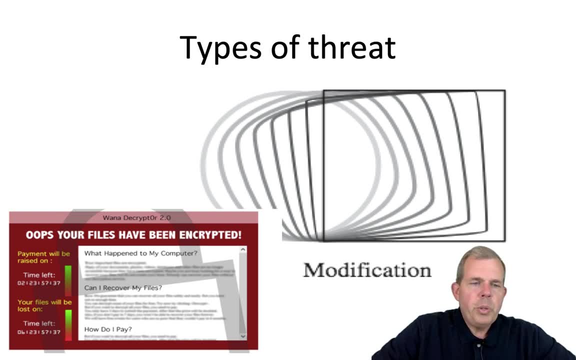 vulnerable to it. and of course, the threat is best avoided by updating your systems and having a good file backup. So even if your computer does get completely unusable, of course you have one or more of these in your desk, correct? So that way you can just restore from backup and the threat goes away. 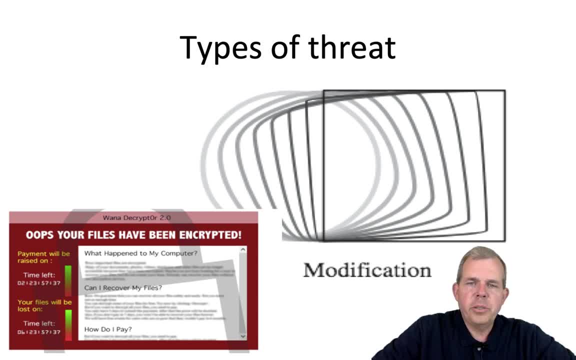 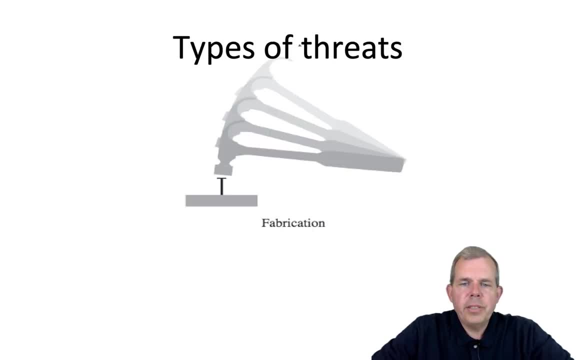 However, most of us don't do the backups, and so we're vulnerable to a modification of the data that we have. Another type of threat you might come across is a fabrication, And so this is different than modification, because you might have the ability to. 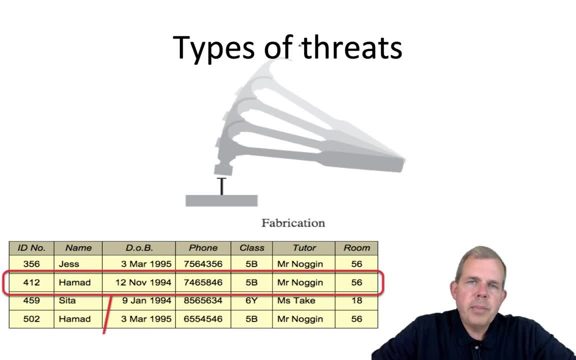 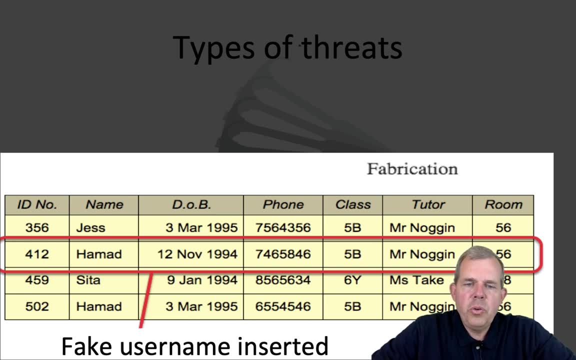 And so this is different than modification, because you might have the ability to slip a new account, for instance, into a computer system. So if we were to insert a new user in the user's table of a database and that had the correct privileges to do administrative work, 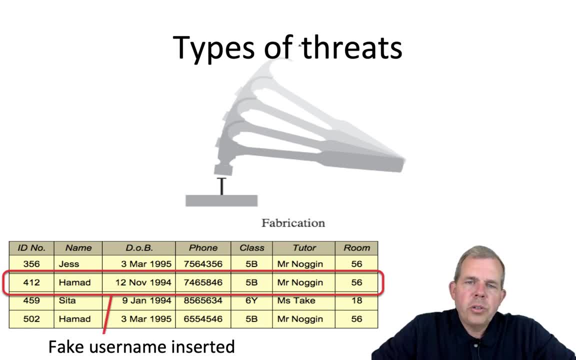 you've got a fabrication threat, Or you might insert some new data that would modify the orders of a system, or a new transaction in a bank account, or any number of pieces of data that the user, the hacker, invents to create an advantage for himself. 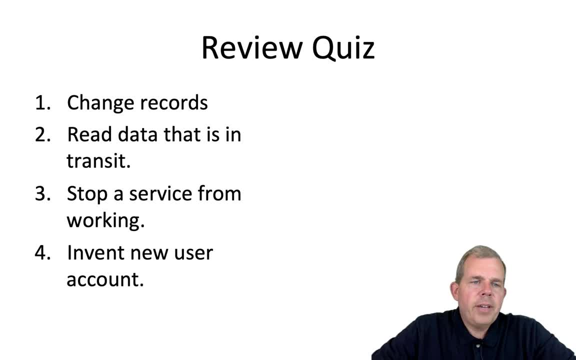 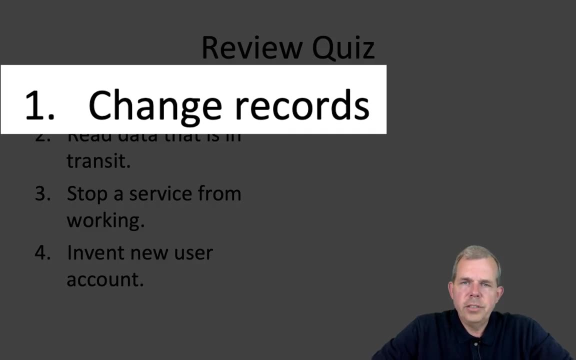 All right, so let's take this quiz that I promised you. I've got four different things here on the screen, and your idea is to identify which kind of attack or which kind of threat is at stake here. So let's talk about number one. that says change records. Do you remember the four types? Well, 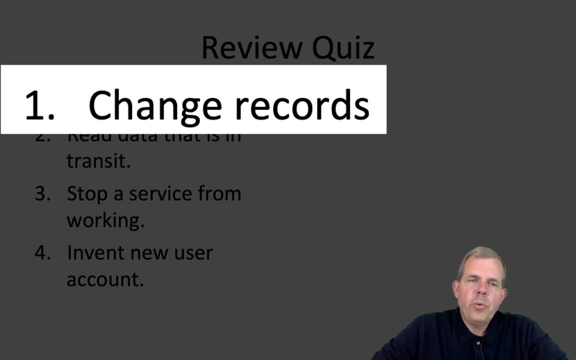 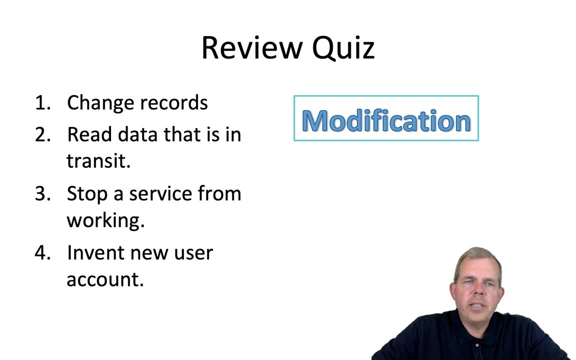 let's go back to the video Rewind, if you have to, to see which one of those four types is at stake. It might be So. if you chose modification for the first answer, you'd be correct. So changing a record is modifying the data that a person has. How about number two reading data that is in? 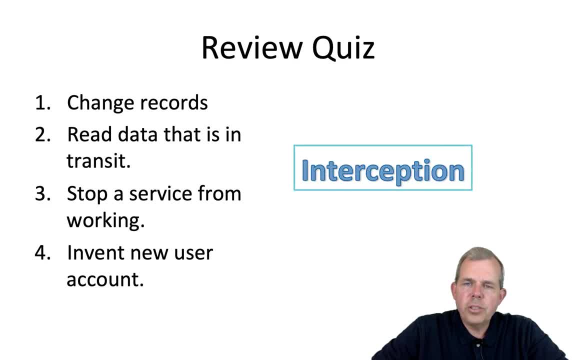 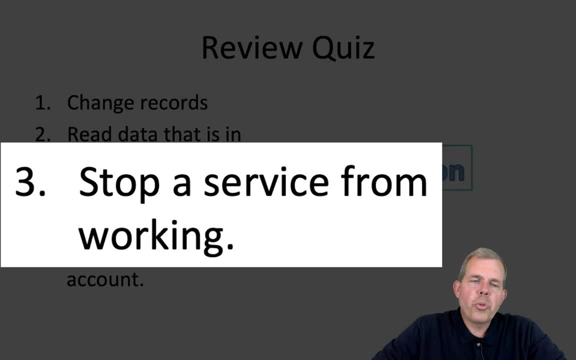 transit. So it's on the network and you intercept it. That's the correct answer. Yes, you interception is reading data that is unauthorized. How about number three, then, stopping a service from working correctly? That would be called an interception. 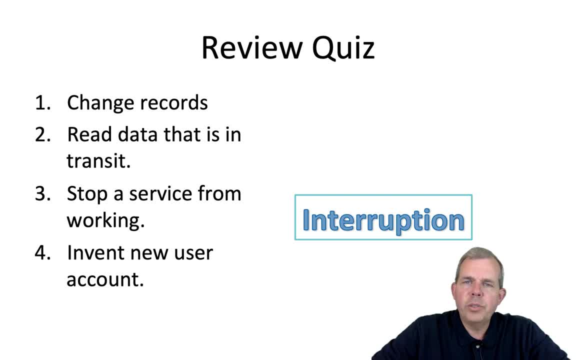 Interruption attack, or some people would call it a denial of service, which is a specific type of interruption. You could simply crash a system so that it comes to a halt. That would also be hardware failure or something, but it's an interruption to normal service. Then the last. 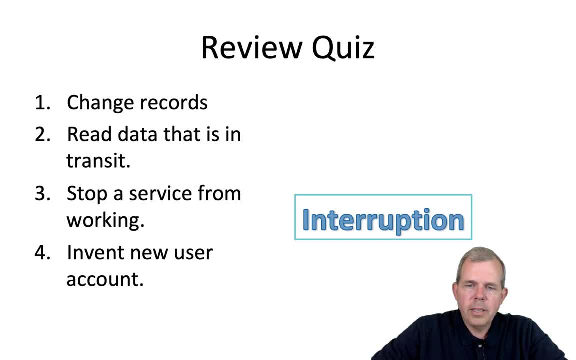 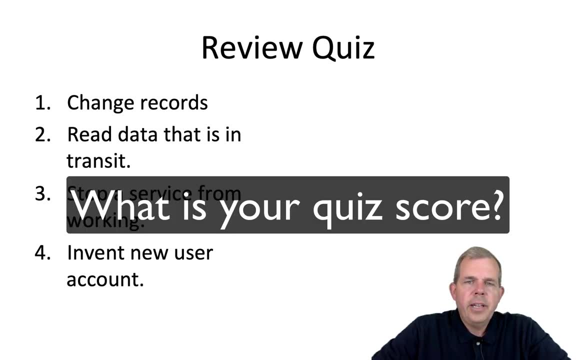 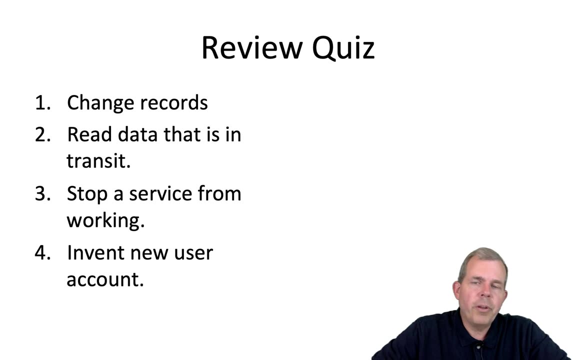 is inventing a new user account. What would that be? If you answered fabrication, then yes, you are correct. So now rate yourself one through four on the quiz. If you got a four, congratulate yourself, And then you can download a file from a link in the description. Run this program on your. 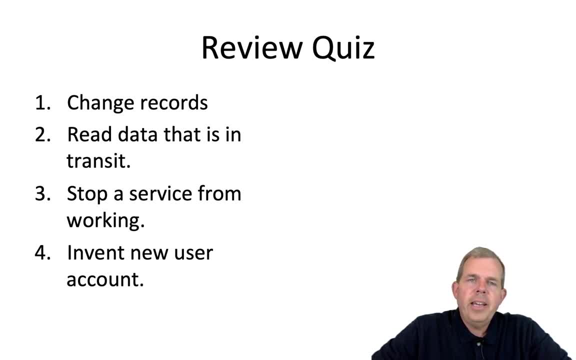 computer and it will play some nice music for you. And, of course, your computer is completely secure. Always accept all kinds of permission requests from anything that I give you. Now we've been doing the class here. We looked at vulnerabilities and threats In the next video. 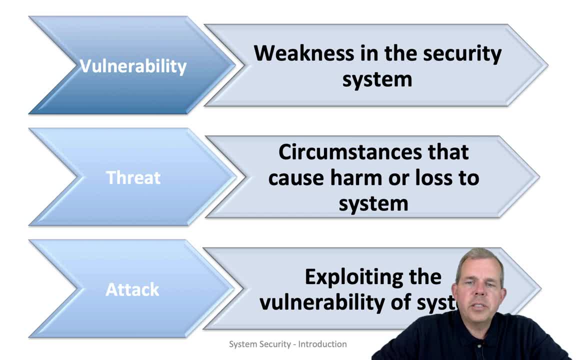 I'm going to show you it's going to be different types of attacks and how we can exploit the vulnerabilities of computer systems. So thanks for watching.